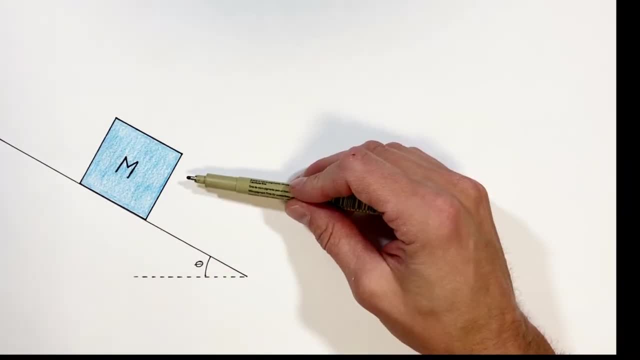 is what we call the critical angle, And today I want to go through and derive an equation for the critical angle of this block against the hill as a function of the coefficients of friction and any other variables that might play a role in this problem, To get a better understanding of what's going on in this problem. 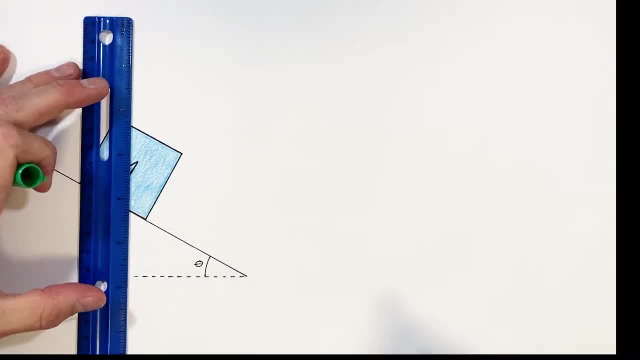 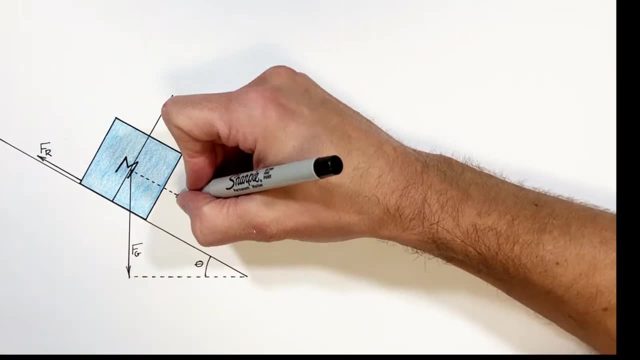 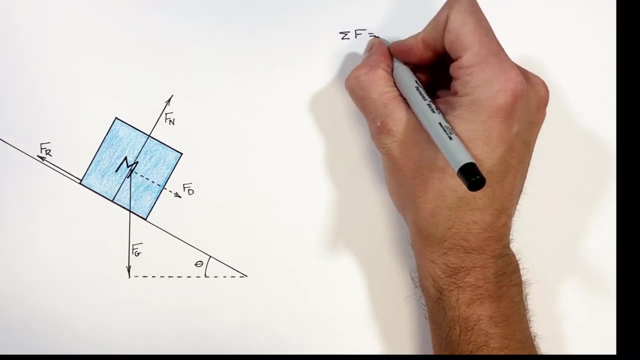 we need to draw a free body diagram for our block on the hill In order to determine the critical angle at which this block is going to slide. we need to take a look at Newton's second law, And what I want to do is look at Newton's second law. 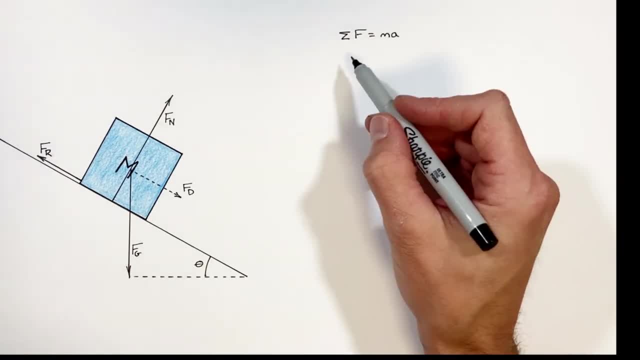 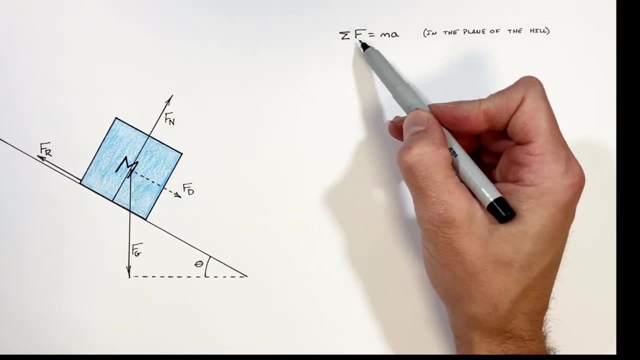 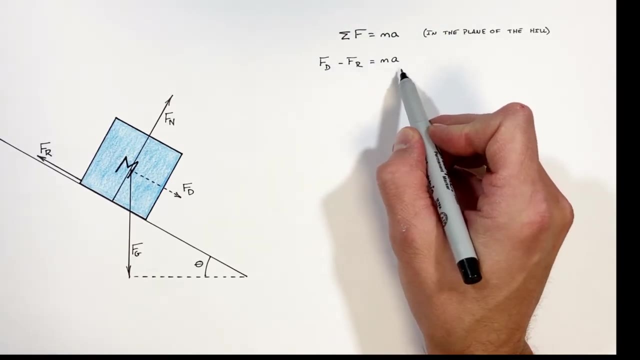 not within the y-axis or the x-axis, but I want to look at Newton's second law within the plane of the hill. So taking our forces and plugging them in here into the sum of all forces side of Newton's second law, we're going to have the force down the hill. minus friction equals mass times. 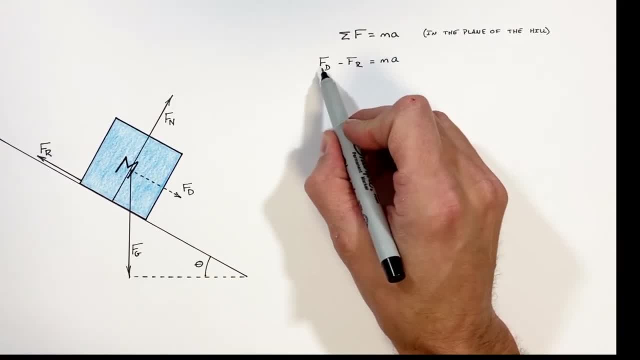 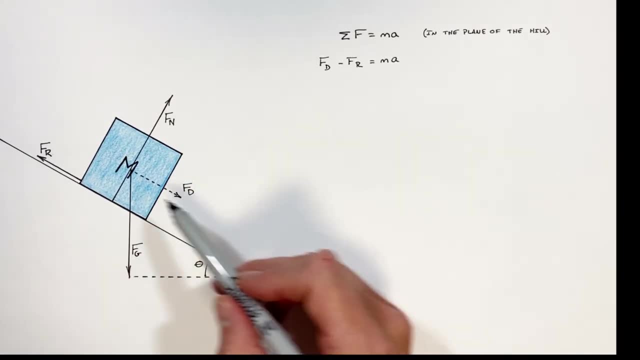 acceleration. Now the reason I've structured these forces where we have one minus the other is because the two forces are in opposite directions. So we're saying the force down the hill is in the positive direction and the friction force is going to be up the hill in. 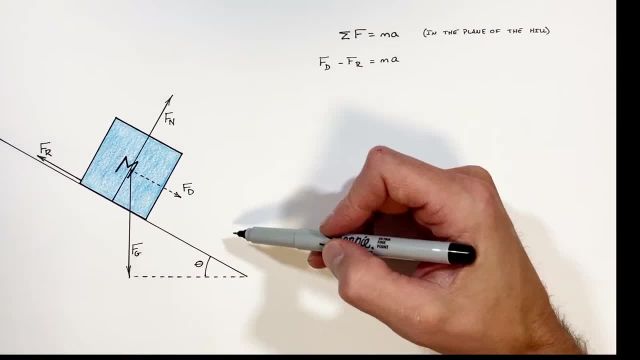 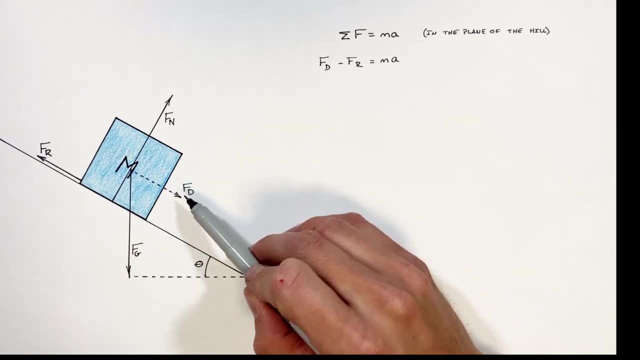 the opposite direction, So I'm saying it's in the negative direction. Now remember, in this problem we're solving for the x-axis and the y-axis are in the opposite direction, So we're solving for the angle at which this block just starts to slide down the hill, or really right at that instant. 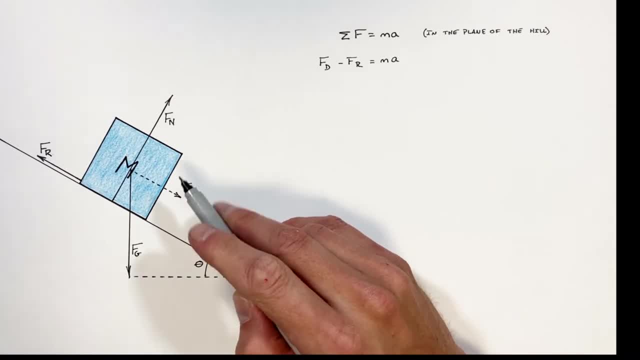 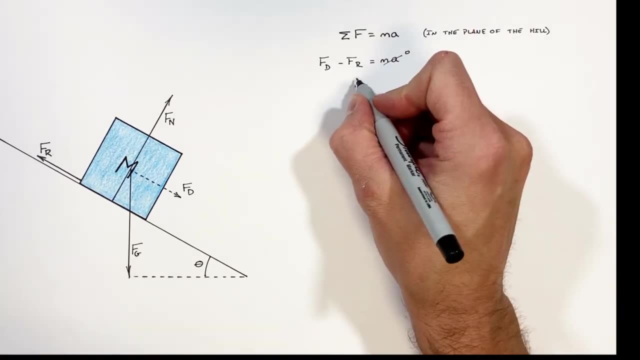 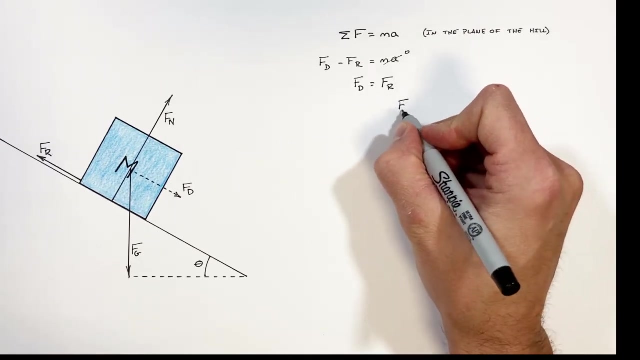 when static friction breaks free and it becomes kinetic, And right at that moment the acceleration is zero. So ultimately, what this means is our force down the hill is equal in magnitude to the friction force. Next, let's expand out these two terms. We know the force down the hill is given by mg sine theta and the friction force is given by. 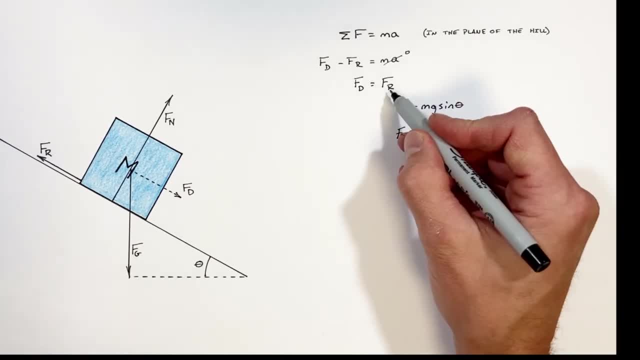 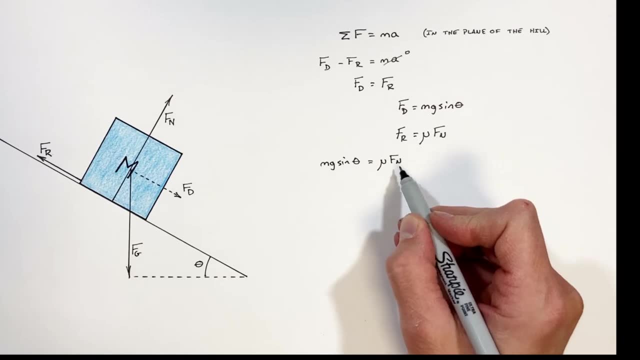 mu Fn. So substituting these terms into our equation will give us mg sine theta equals mu Fn. Now realize the trick in this problem is realizing that Fn can also be expressed as a function of the angle of the hill and the mass of the block. So substituting this 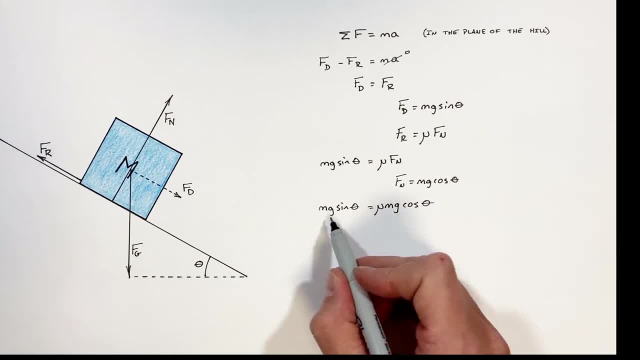 term in here we get this term and you'll see mg cancels out on both sides. And if we want to relate mu to theta, we need to combine the cosine and the sine And we're left with this. mu is equal to the tangent of theta, Or rearranging this for theta we get.